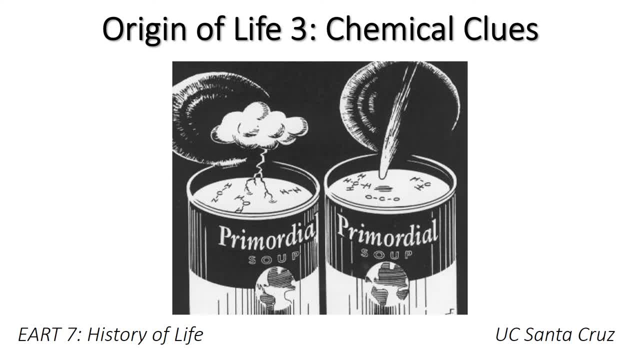 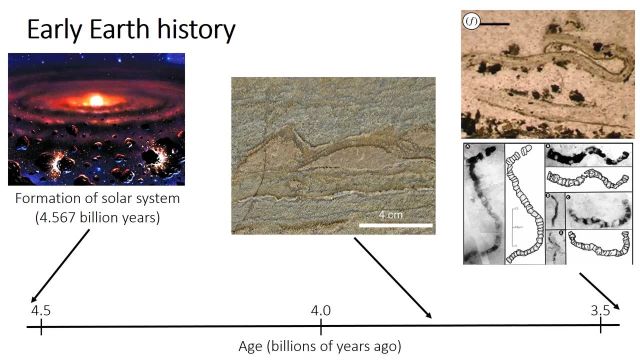 Hello again and welcome back to the final topic in our discussion of the origin of life. These short videos will discuss a different type of evidence: chemical evidence for early life on Earth. So just to recap the evidence so far, the solar system and Earth formed a bit over 4.5 billion years ago. 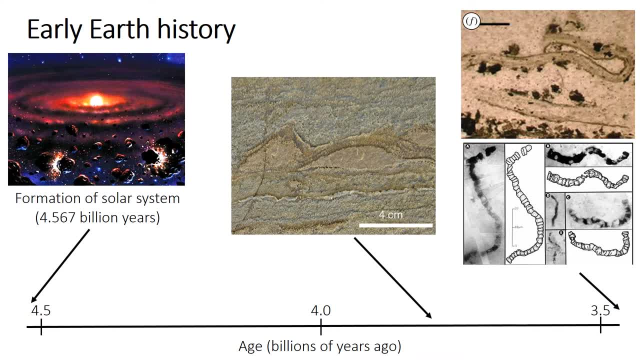 but there's not much evidence and no sedimentary rocks for the first 700 million years. We discussed before some possible but also very controversial stromatolites from Greenland that are about 3.7 billion years old, and we also discussed possible microscopic fossils of bacteria. 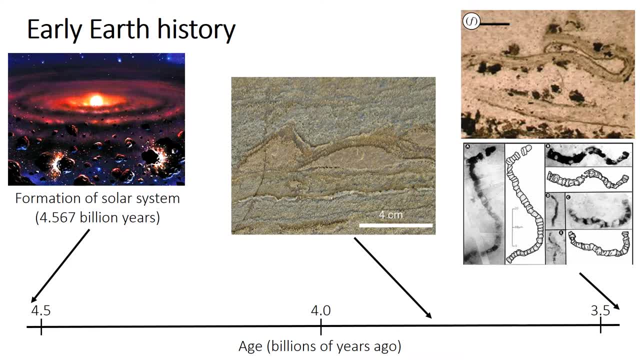 that are about 3.4 billion years old. While some of these evidences are still debated, there are actually a variety of other lines of evidence that do suggest that life was present by this point, around 3.4 or 3.5 billion years ago. 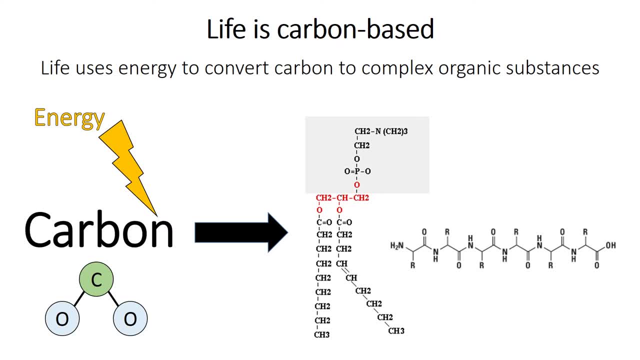 Well, so far Now, we've discussed physical structures as evidence for life- stromatolites, microfossils- but perhaps scientists could instead use chemical evidence. Well, on Earth, life is carbon-based, which means that the molecules that form all living things 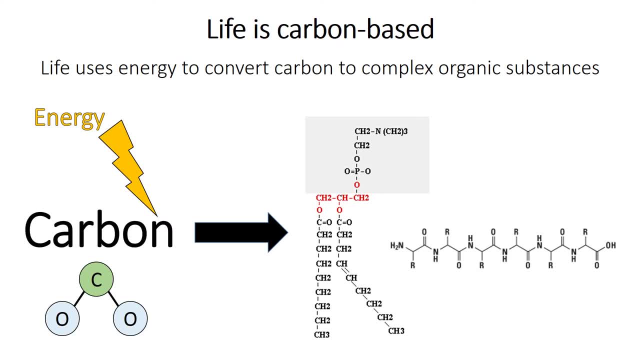 are made up of long chains of carbon atoms, with some other elements like nitrogen or phosphorus in there as well. Living organisms build these molecules by using energy, either from sunlight or from chemicals, to convert the energy. So we can say that the carbon atoms that are made up of carbon atoms are made up of organic carbon that's in the water or in the air. 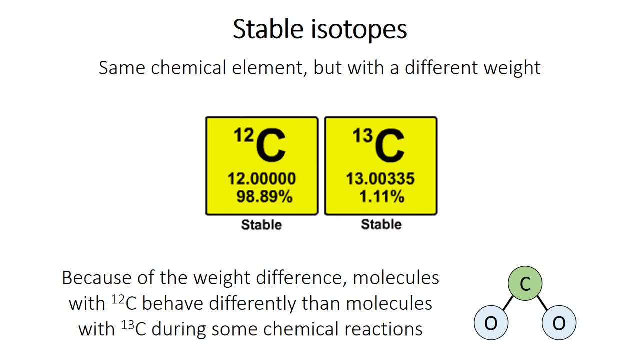 There's actually two different types of carbon atoms. Well, there's three types, if you include the radioactive carbon-14.. These different types are called isotopes, which means that they're the same chemical element. they're all carbon, but they just have a different weight. 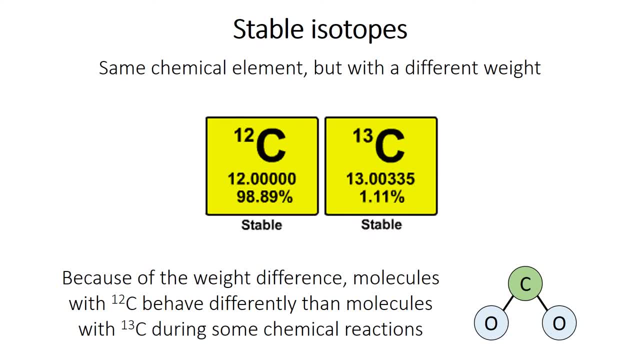 The carbon that has an atomic weight of 12 is the common form. It's nearly 99% of all carbon atoms, But there's also an isotope of carbon that's called isotope. It contains one extra neutron, So that means it weighs 13 units instead of 12.. 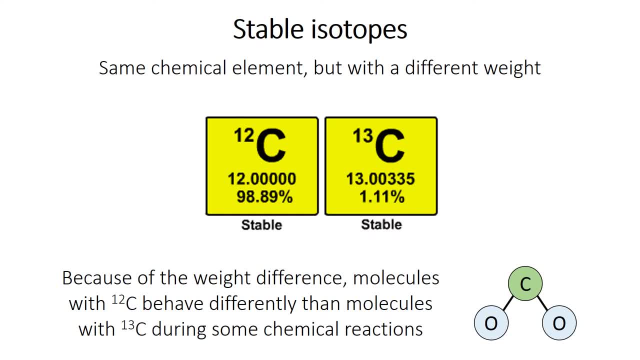 Well, this weight difference means that molecules containing carbon-12 behave differently during chemical reactions from the molecules containing carbon-13.. In particular, the chemical bonds between carbon-12 and other atoms are just a tiny bit easier to break apart than the chemical bonds between carbon-13 and other atoms. 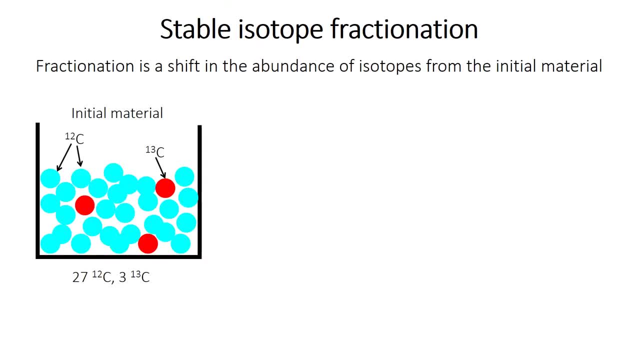 Well, because some molecules are a little bit easier to break apart, this can cause the abundance of the different isotopes- carbon-12 and carbon-13, to change from the initial material to the new substance that's made from those atoms. This change in isotopes is called fractionation. 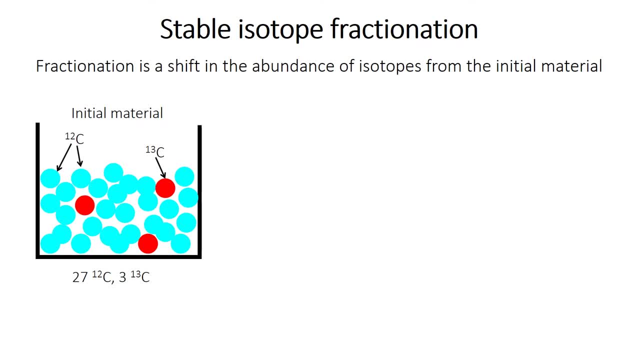 So imagine you have some initial material- in this case let's just say carbon, contained in seawater, and it has some amount of carbon-12 and some amount of carbon-13. The numbers here are just for illustration, just to show, Well, when an organism breaks apart those carbon molecules. 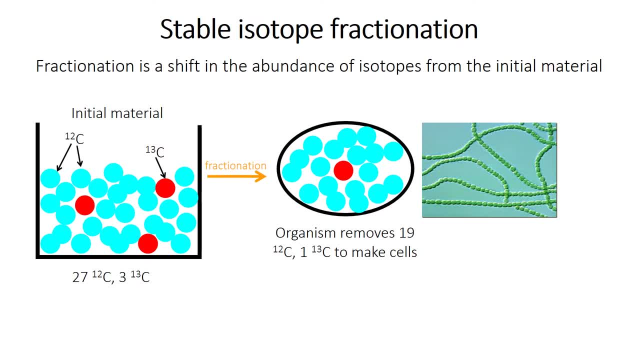 and makes new organic molecules out of them. the organism takes a little bit more carbon-12 than was initially present in the seawater and therefore a little bit less carbon-13. So our organism has more carbon-12 than the initial material did. 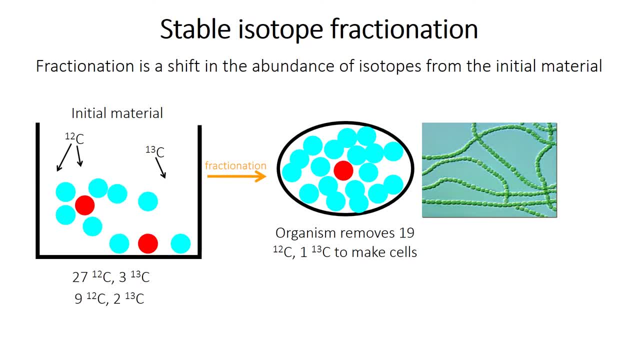 Well, as a result, the leftover seawater carbon has less carbon-12 and more carbon-13 than initially did. When a rock is formed from that seawater, there's no fractionation, it just records the composition exactly as it is. 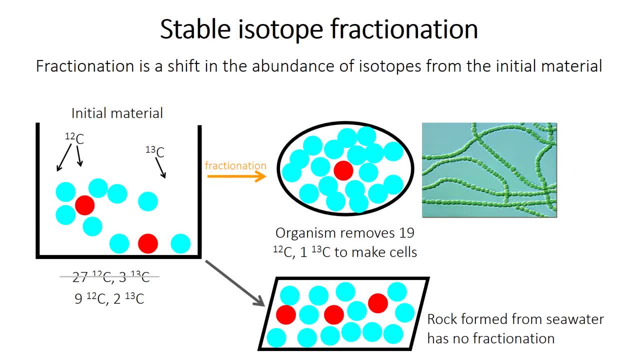 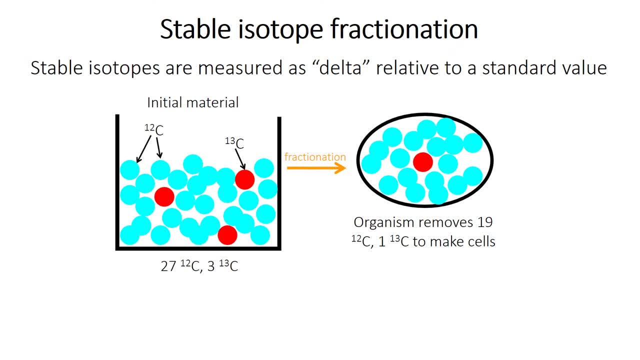 so the abundance of carbon isotopes is the same as the seawater Well. in reality it's super hard to count the actual numbers of each atom, of each isotope, So they're actually measured in a relative sense compared to a standard material. 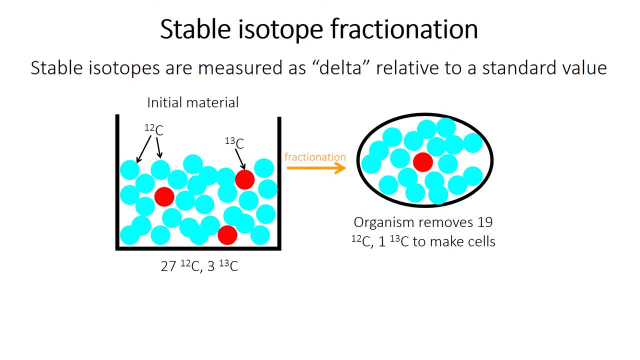 and this is written with the Greek language letter delta. So if the delta-13C- as we call it, the delta-13C- value is positive, that means that the material has relatively more carbon-13 than our standard material does. 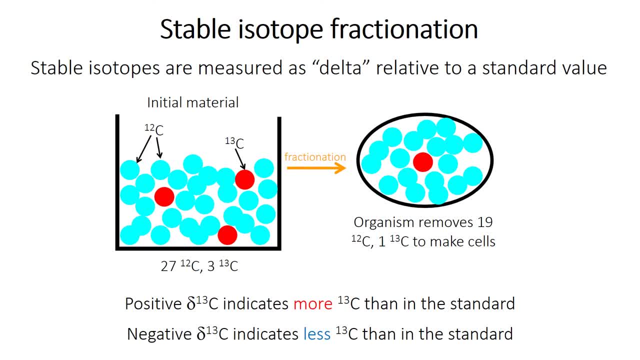 and a negative delta-13C value means that the material has less carbon-13 and therefore more carbon-12 in a relative sense, compared to our standard material. Negative values are sometimes also called depleted and positive values are sometimes called enriched. Well, because organic matter contains relatively more of the carbon-12,. 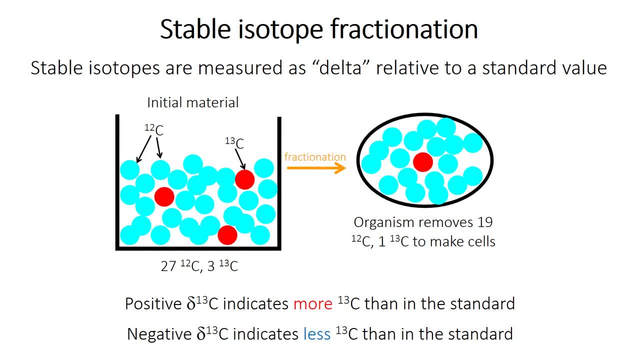 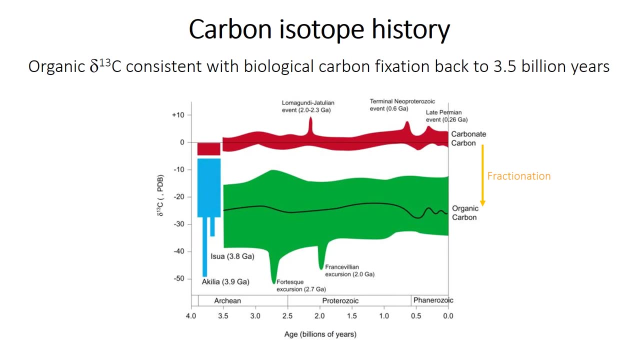 due to it being easier to break apart those carbon-12 molecules, organic matter would have a negative or depleted delta-13C. So geologists have measured the carbon isotopes, the delta-13C, from rocks and from organic matter throughout Earth history. 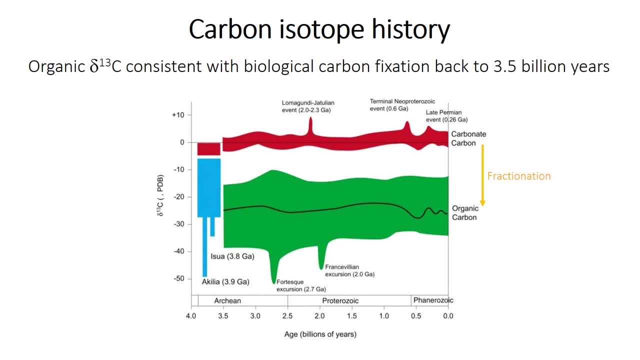 and this graph shows time going from left to right, from about 4 billion years ago until today, at zero. The vertical axis shows the carbon isotopes, which is measured in parts per thousand, because the differences are normally pretty small. Organic carbon molecules typically have values of between minus 20. 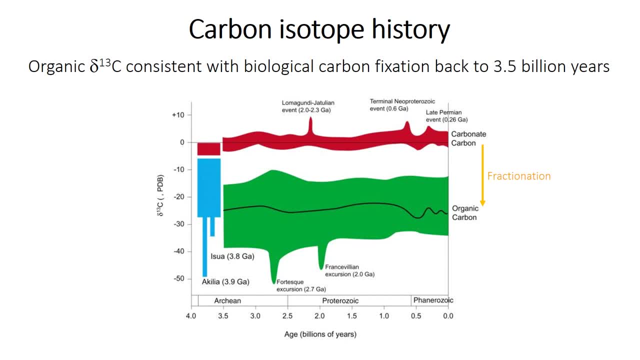 and minus 30 parts per thousand. That's shown by this green band and that indicates that there is about 20 to 30 parts per thousand less carbon-13 than there is in the standard reference material Rocks that form from the seawater. 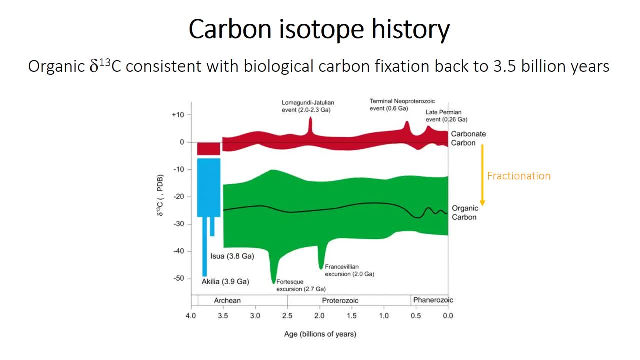 in this case what's called carbonates, normally have slightly positive carbon isotope values, because that's what's left over after removing a little bit of the carbon to make organic matter. So the isotopes of organic carbon are pretty similar all the way back to 3.5 billion years ago. 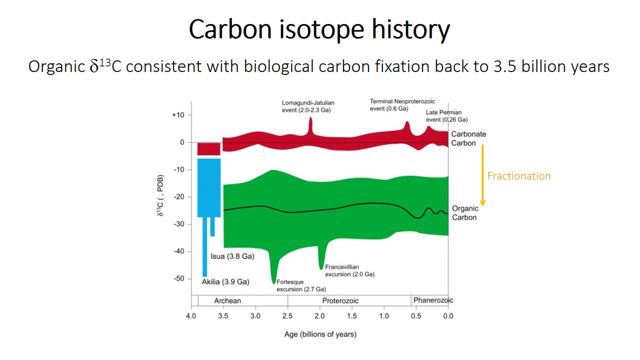 and that's consistent with life producing that carbon. But we're actually today going to talk about some carbon isotope measurements from Greenland, especially from this place called Achillea, dating to 3.8 or 3.9 billion years ago. 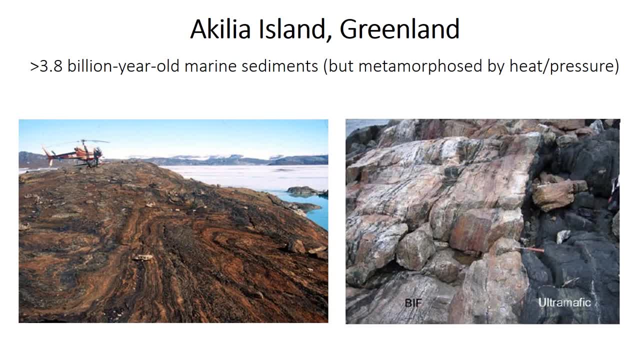 So back to Greenland. We've talked about the possible stromatolites from Greenland, but this is a nearby, different place called Achillea Island. This island contains rocks interpreted as marine sediments, although they've been subjected to high heat and high pressure since they formed.